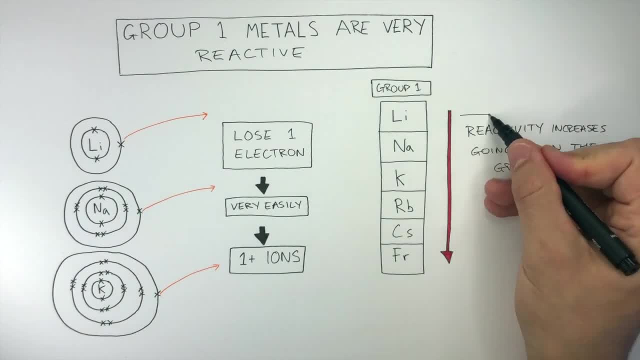 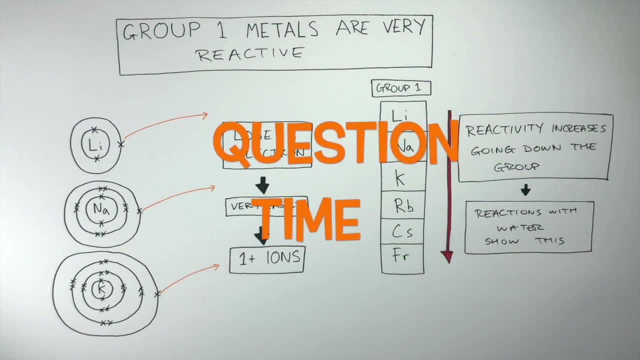 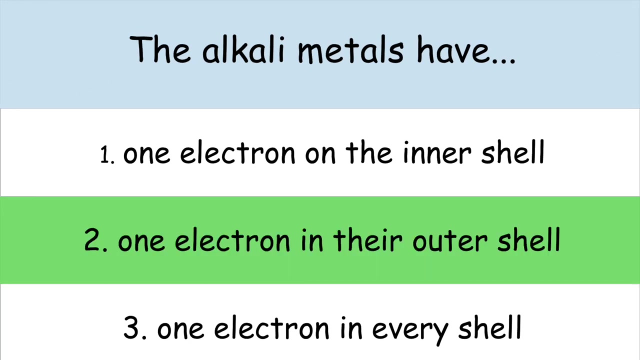 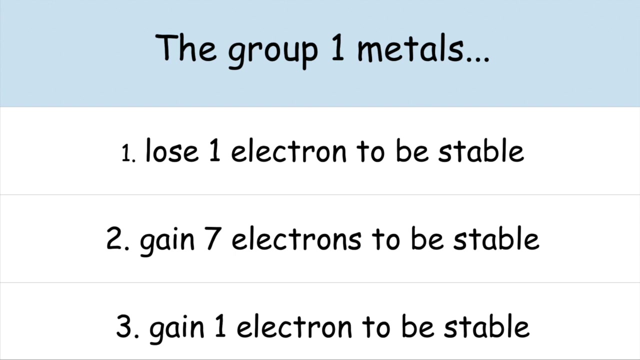 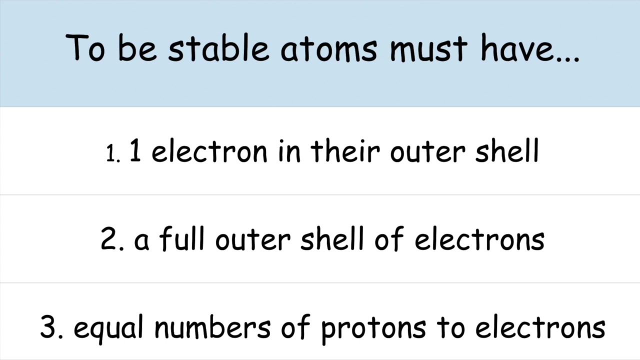 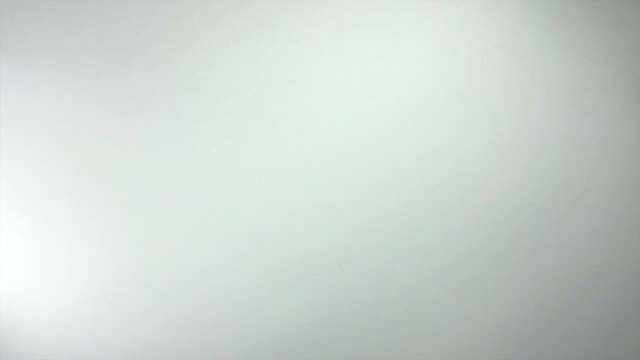 The reactivity increases going down the group And we're now going to see how reactions with water show this. It's question time. Attempt these questions to check your understanding. Let's first go through the safety precautions when reacting alkali metals with water safely. 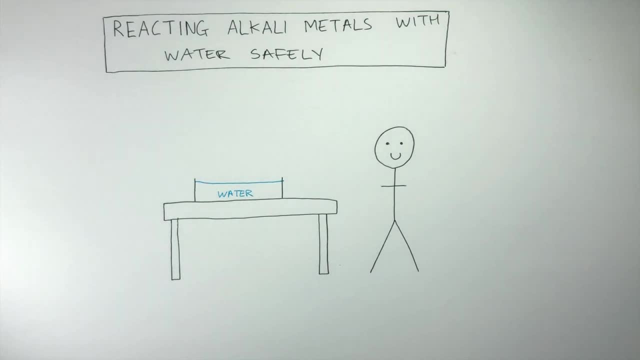 As these reactions are so vigorous and have the potential to be quite dangerous, the teacher has full responsibility for this reaction. A trough of water is placed on top of a smooth surface such as a table, and placed behind the safety net. The pupils are safely behind the screen and are protected from the glass trough potentially breaking if the reaction is too vigorous. 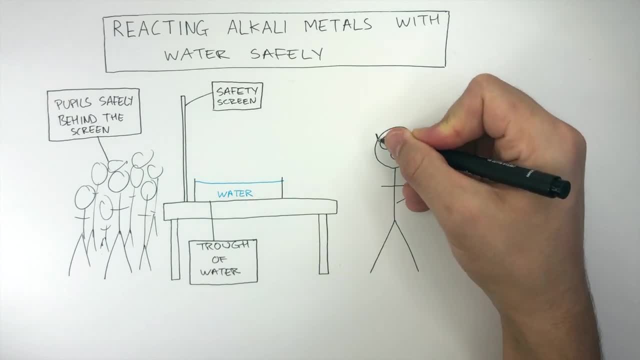 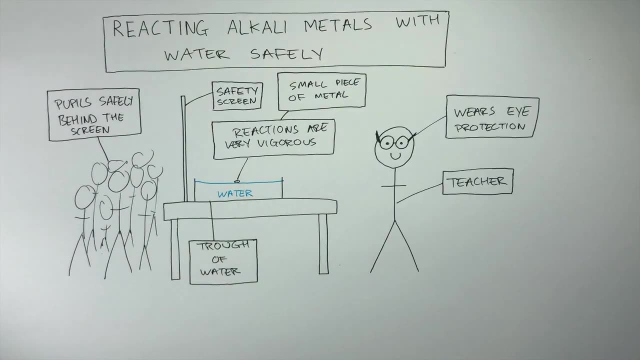 The eyes must be protected, so the teacher wears eye protection. The reactions are very vigorous, so a small piece of metal must be used. The teacher must do the experiment, as the reaction has the potential to be quite dangerous. The teacher must do the experiment, as the reaction has the potential to be quite dangerous. 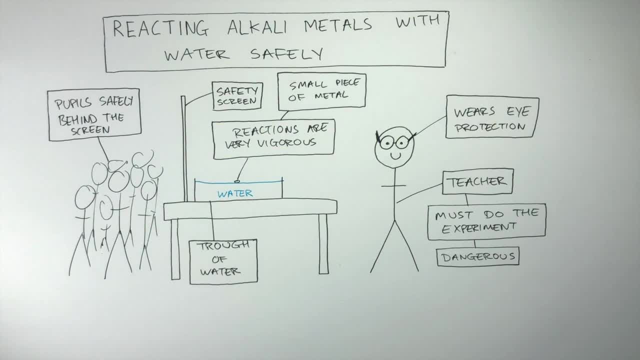 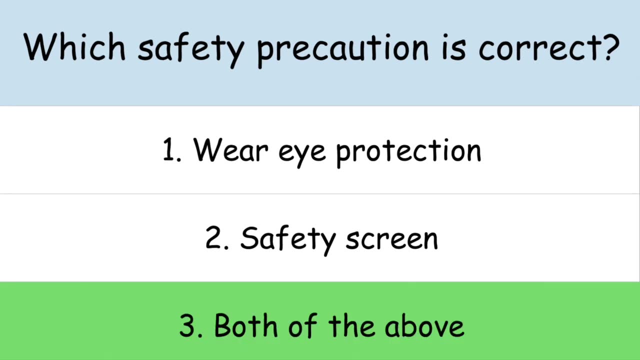 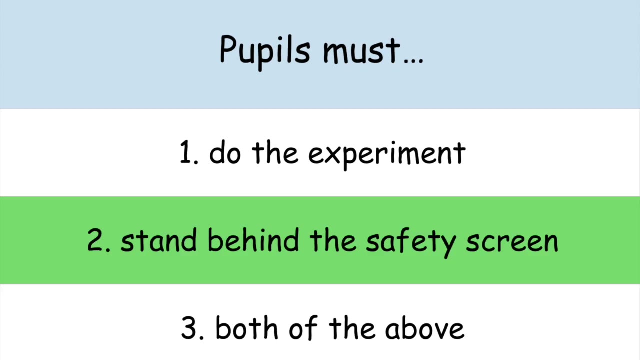 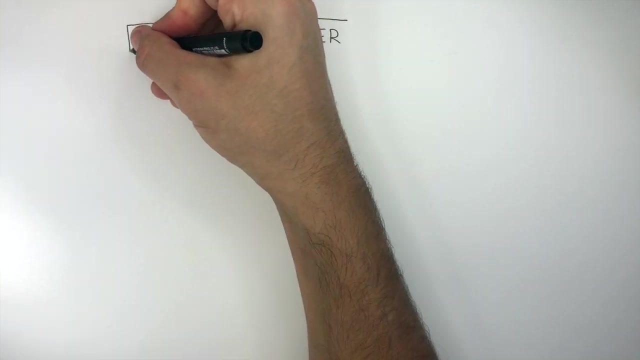 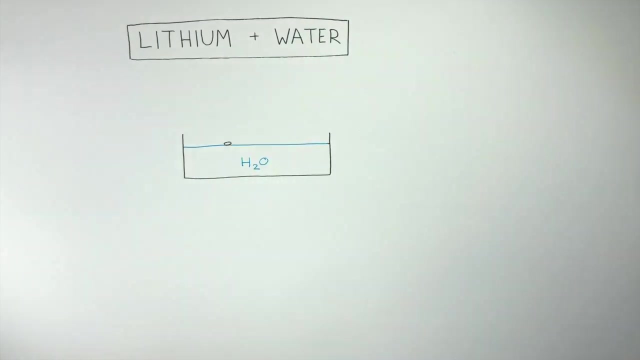 It's question time. Attempt these questions to check your understanding. The reaction between lithium and water is the least vigorous reaction out of all the group 1 metals: isawa, isawa. This is the glass trough: isawa, isawa, and it is filled with water. the small piece of lithium metal is dropped into the water, where? 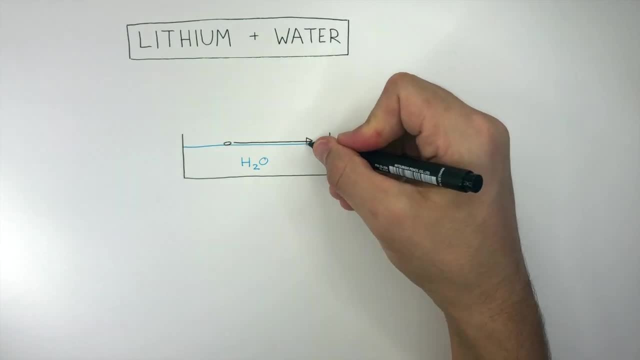 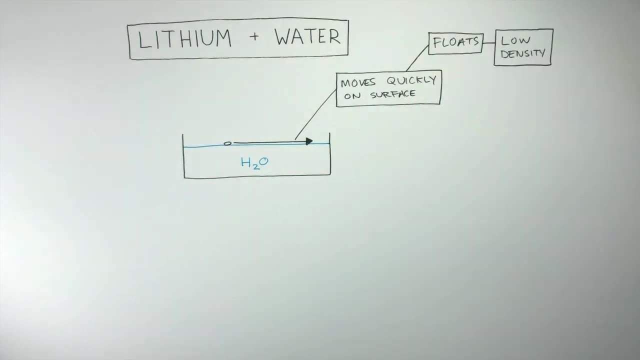 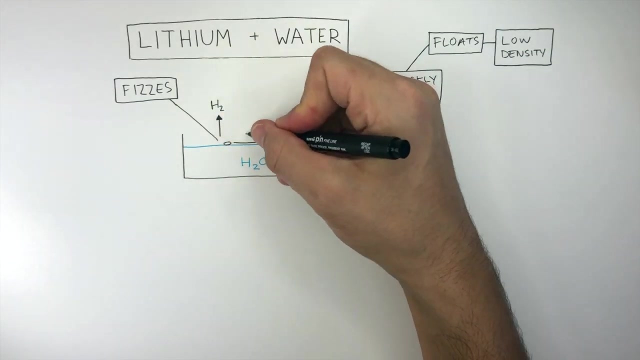 it reacts very quickly. the arrow shows how the lithium moves quickly on the surface and it floats because it has a low density, lower than water. the lithium fizzes as it reacts with the water. this is due to hydrogen gas being given off, if you ever see fizzing in any chemical reaction. 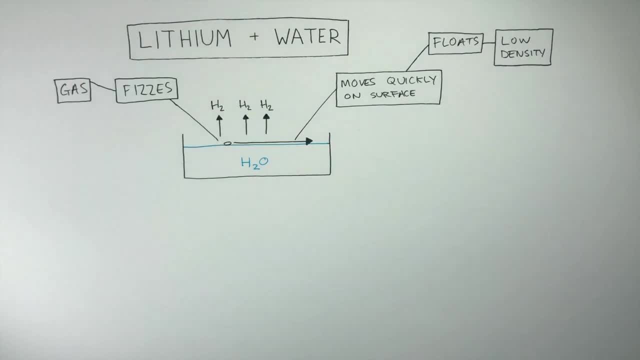 this means a gas is being given off, and in this case it is hydrogen. hydrogen gas is a product. whenever a group, one metal, reacts with water, the word equation for this chemical reaction is lithium plus water goes to lithium hydroxide and hydrogen, the aqueous lithium hydroxide formed. 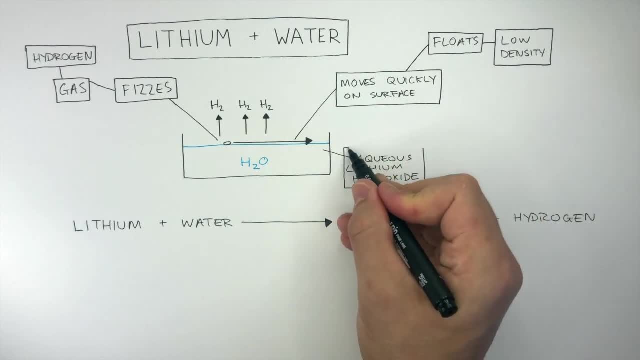 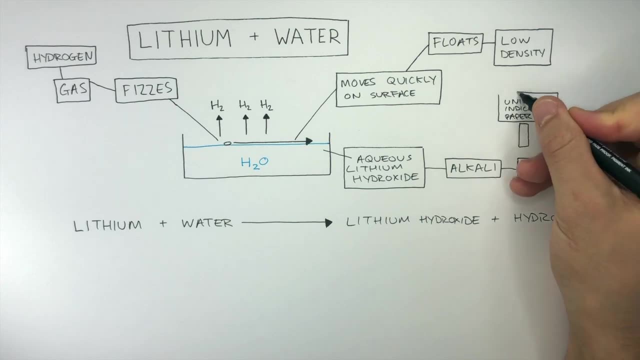 is just lithium hydroxide dissolved in water. it is alkali as it has a high ph and causes universal indicator paper to turn purple. this is the case for all metal hydroxides. the symbol equation is li s for solid plus h2o. alpha liquid reacts to form. 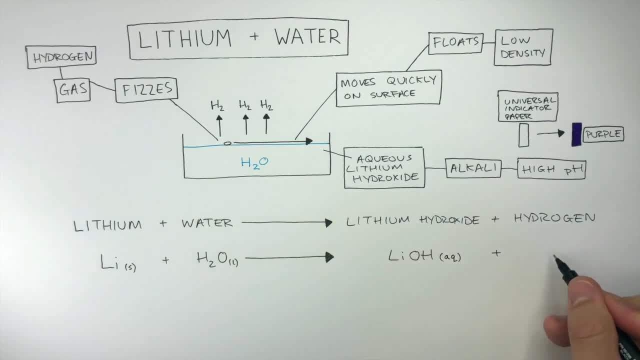 li oh h, aq for aqueous plus h2, g for gas. this equation is not balanced. to balance this, we're going to mark it down to, let's say, 7 for aqueous plus h2ados. but instead of letting it happen for just a moment, we're going to everyhões. president inrang, for every Lindgley was weighing that down. 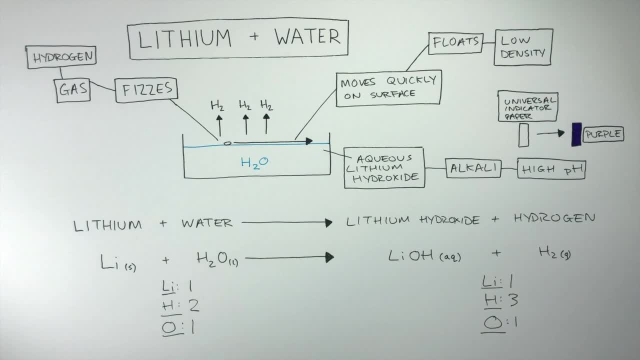 so let's say this: iron was in a both now ethyl lithium when, Carrie, if we were to add 4 li in at and negative charge to aqueous plus aqueous is exactly a very high Geschlechtra freedom if you were writing down a value for aqueous, true, we could write down a value as mod wheel if we were. 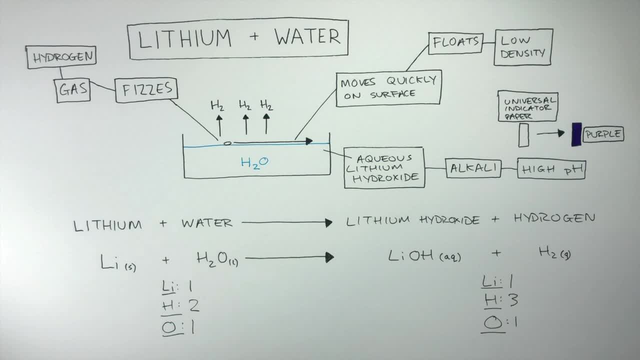 to write down at andkim. breaking it down to observability, which will be at mu comma zero north, AND there is one oxygen atom. We can see this reaction is not balanced because there are two hydrogen atoms on the left and three hydrogen atoms on the right. Therefore, we now need 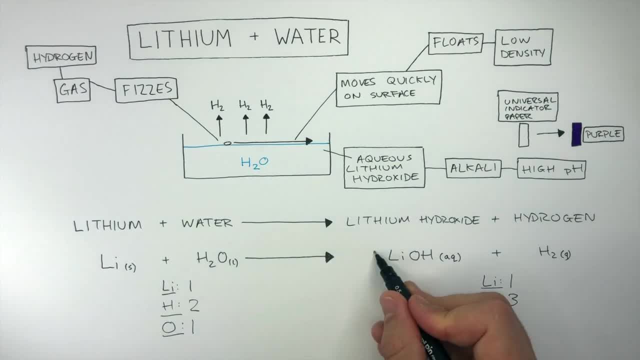 to balance this. To balance this, we put a big 2 in front of the LiOH. This means there are now two lithium atoms, four hydrogen atoms and two oxygen atoms. on the product side, We now put a big 2 in front of the H2O, so there are four hydrogen atoms on the left. 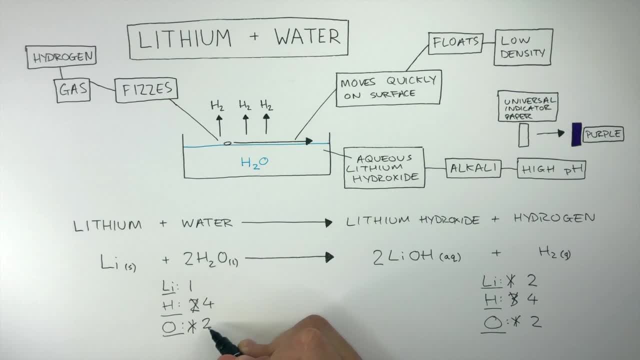 and two oxygen atoms on the left. The hydrogen and oxygen atoms are now balanced. Finally, put a big 2 in front of the lithium atom on the reactant side, so there are now two lithium atoms on the left. This chemical reaction is now balanced. 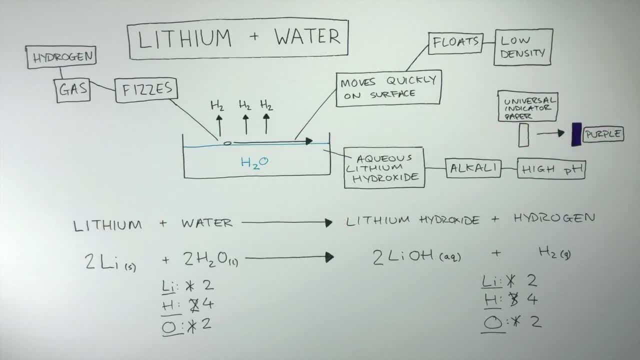 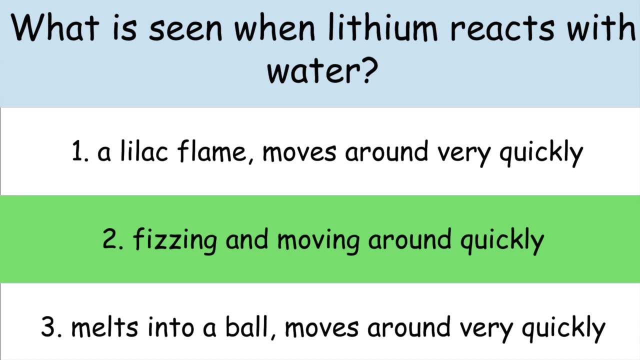 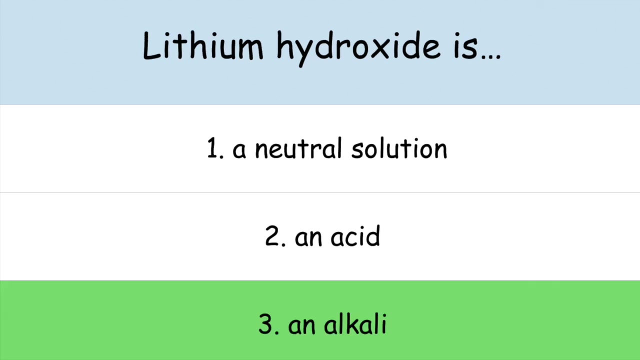 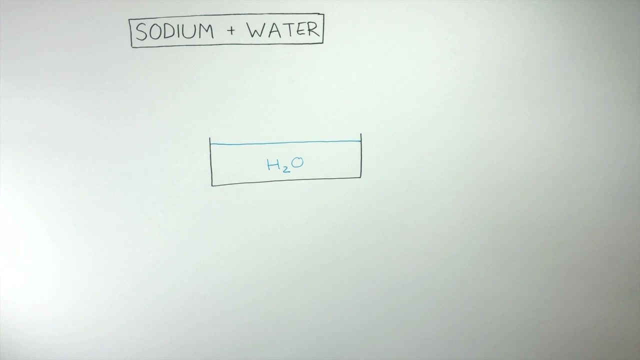 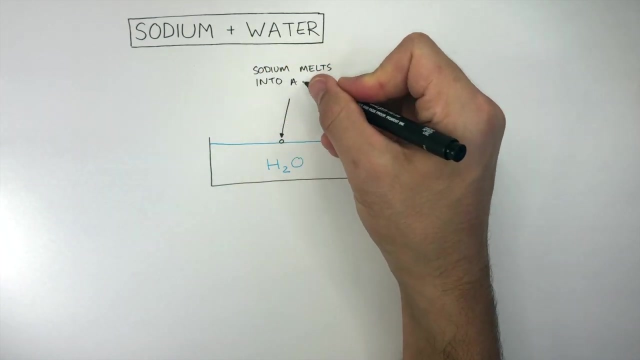 It's question time. Attempt these questions to check your understanding. Sodium reacting with water is a more vigorous reaction compared to lithium. We can see this because when sodium is dropped into water, it melts into a ball and it moves quicker on the surface where it floats, due to its size. 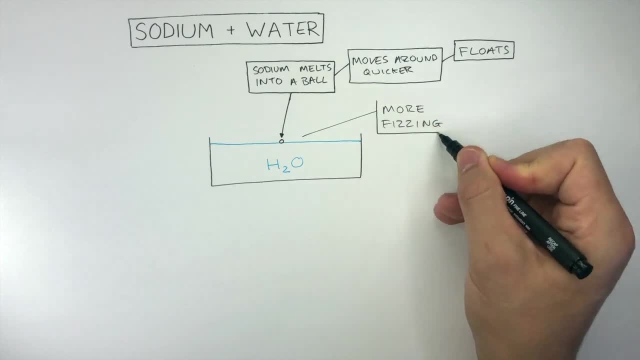 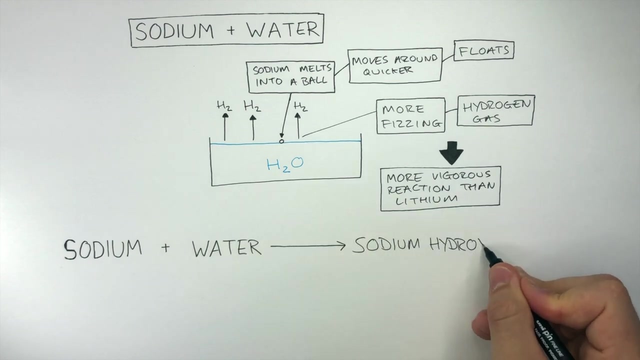 There is more fizzing due to hydrogen gas being given off at a faster rate. These observations show us sodium reacting with water is a more vigorous reaction than lithium and water. The word equation for this chemical reaction is sodium plus water reacts to form sodium hydroxide and hydrogen. 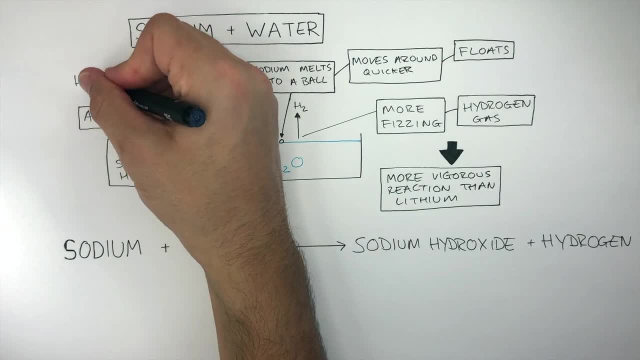 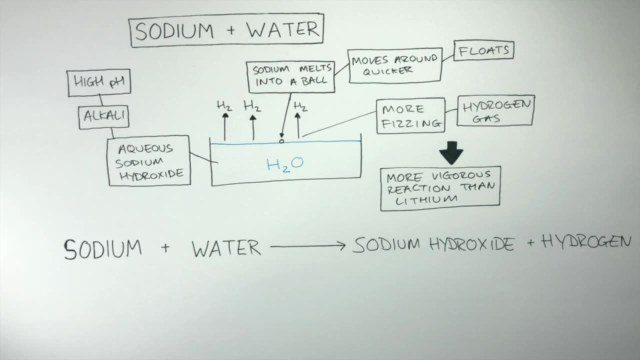 Aqueous sodium hydroxide forms, which is an alkali, so it has a high pH. This can be shown using universal indicator paper which turns purple. Pause the video here to write a balanced symbol equation and the answers will follow. 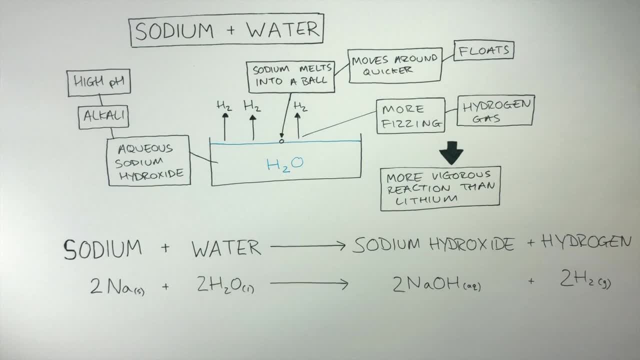 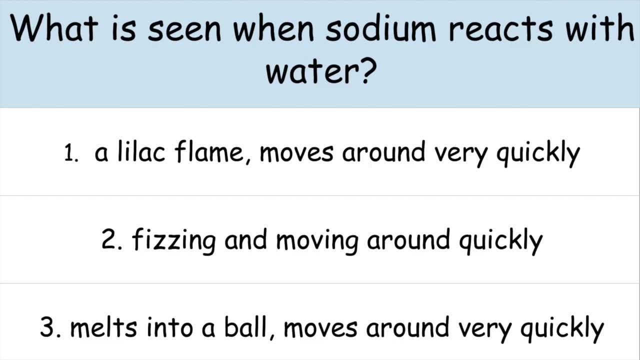 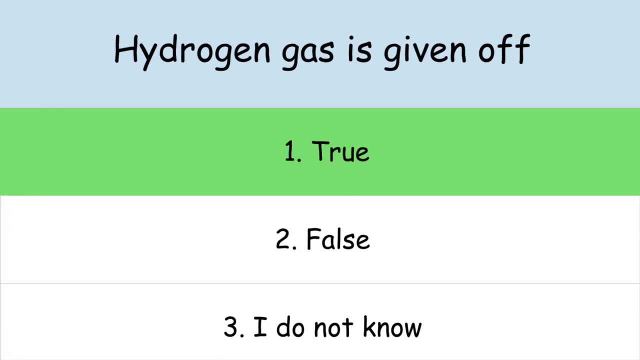 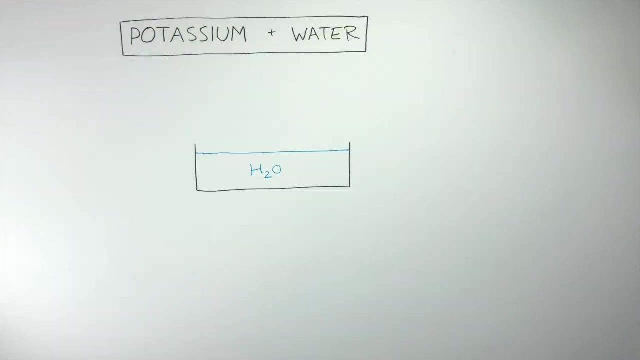 This equation is the same as the previous equation with lithium, except that the metal is now sodium. It's question time. Attempt these questions to check your understanding. Photosynthesis problem. Potassium reacting with water is a more vigorous reaction compared to the очfilmbbt. Habitat bedroom. 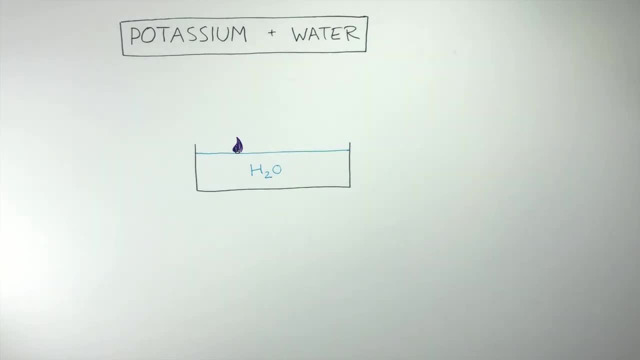 when the potassium is dropped into the water, it reacts immediately, burning with a lilac flame. It reacts vigorously as potassium is turned liquid. Caahan disturb. Bianca D's Pyramid is an öffentlich body called Alkali production. This Alkali process is a power-saving blaze which breaks through Salmian direct universes. 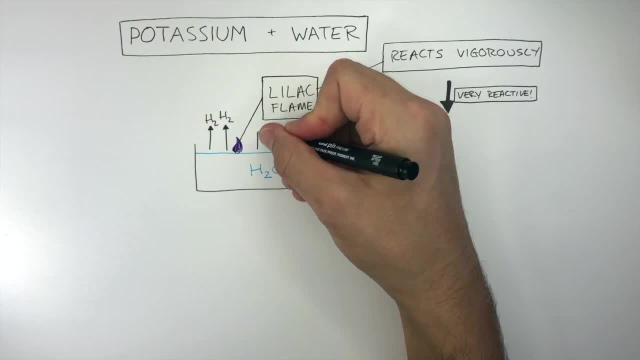 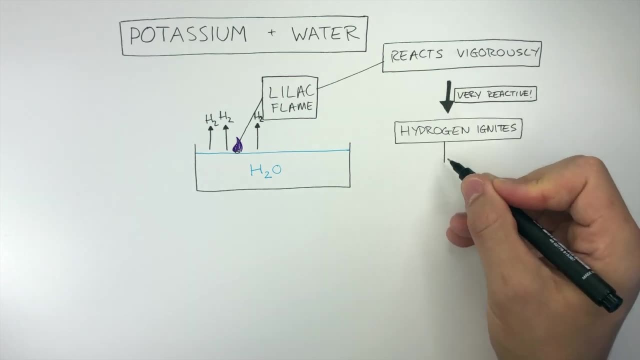 is very reactive. Hydrogen gas is given off and because there is so much heat due to the vigorous reaction, the hydrogen ignites, producing a flame, and it's the potassium ions which cause the lilac colour. The word equation is: potassium plus water reacts to form potassium hydroxide.